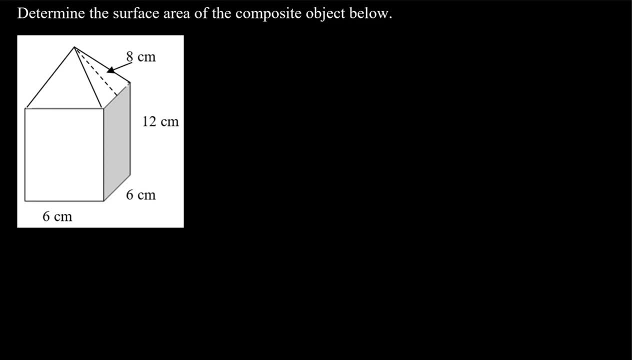 seems to be. it's, it's a pyramid here that's stacked on top of a rectangular prism or a square base prism. so, and it's saying, to find the surface area of the composite object. Well, the surface area. what we want to do is we want to try and 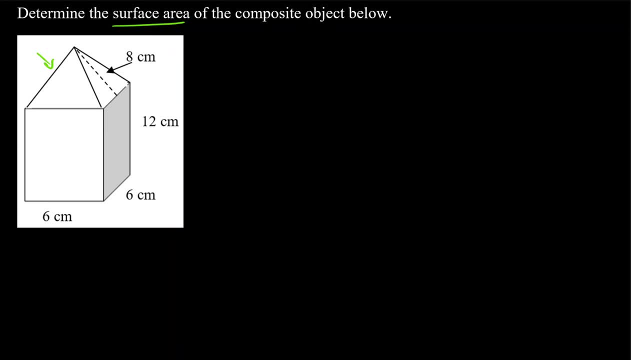 identify all of the surfaces that are showing or that are present in our object. Now, if this was just a regular pyramid and sorry- and a regular prism. when we take one object and we stack it on top of the other, we end up missing or we end up having two of our faces. 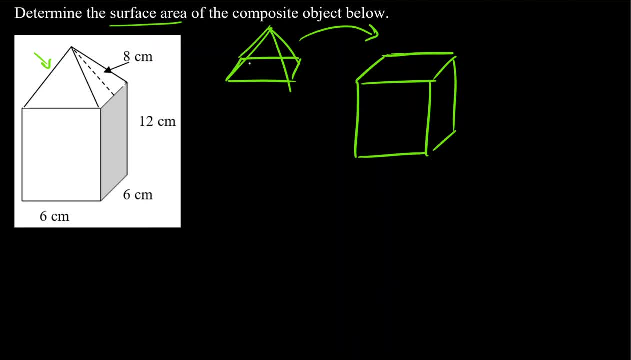 two of the surfaces disappear because of the stacking, so the bottom of the pyramid and the top of the prism are no longer showing. they're no longer like present for us to either paint or cover or whatever we're, for whatever reason why. we're calculating the surface area so we can't. 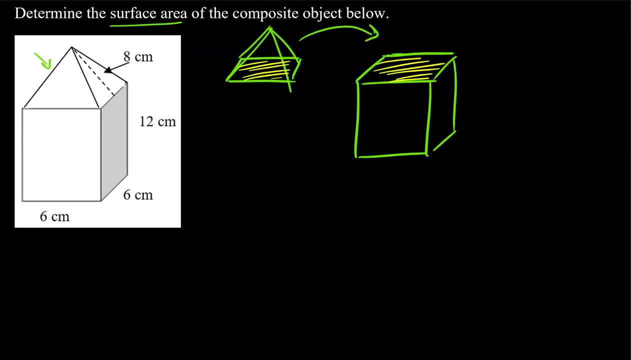 take those sides into consideration. well, what else do we have? what other sides do we have? well, we've got- we still got- our four triangles from our, our pyramid, and we've got the sides of the prism, and then we also have the bottom of the prism as well. so the sides of the prism. hopefully you'll notice. 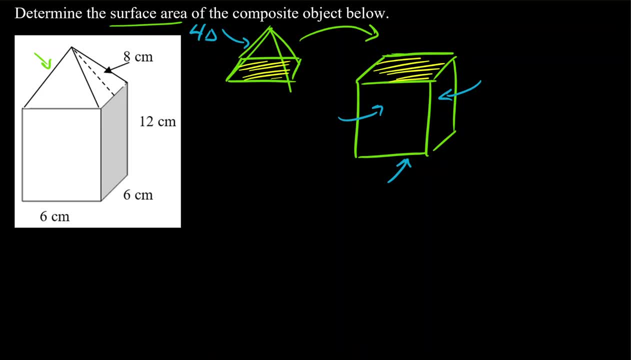 that this is a square based prism, so the bottom is length times length, and the sides, because they share the same height. it's 12 centimeters high and they share the same base, all four sides around this object, all four sides here, at the back and at the side and at the front. they're all the same. so if we want to add up, 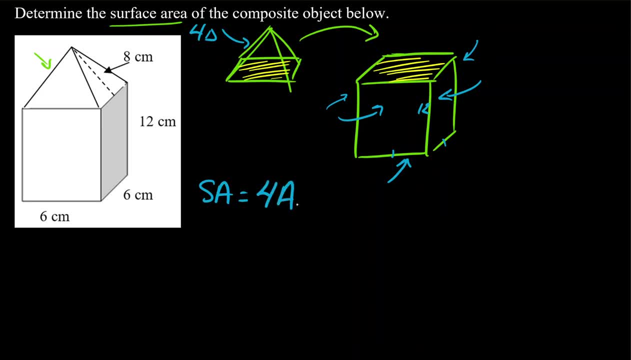 the surface area of this object. it's the four areas of the triangle plus it's the four lateral sides, so the four length times height, plus it's the one bottom and that's length times length, or we could just write that as length squared. so that's the idea. it's the four sides of the triangle. it's the four sides, the lateral. 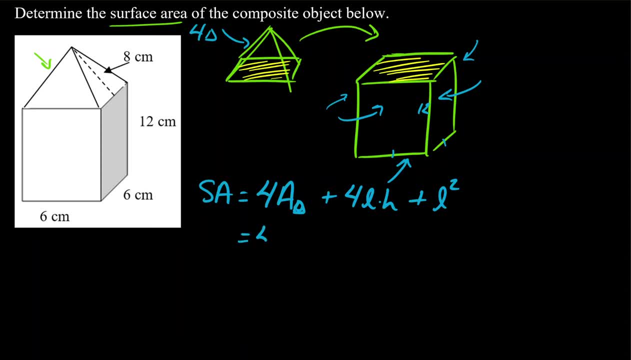 sides of this prism in the bottom. let's go ahead and calculate that four and it's base times height divided by two. so when we look at the base of this triangle, it's six centimeters wide, so six centimeters. the height to the triangle is eight centimeters divided by two. 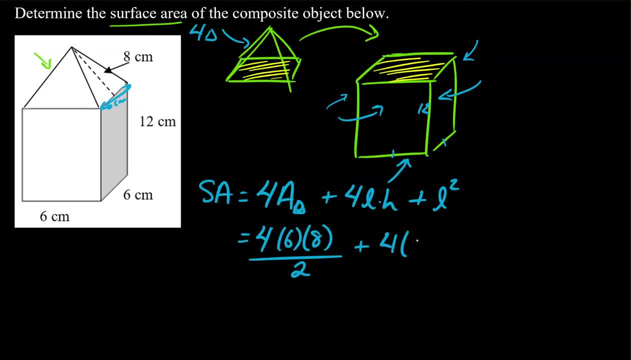 plus four length times height, so six times twelve plus just the bottom is six squared. when i calculate this, i end up getting 420 square centimeters. so centimeters times centimeters is centimeters squared. same thing here, same thing here. so we end up getting 420 square centimeters, perfect. 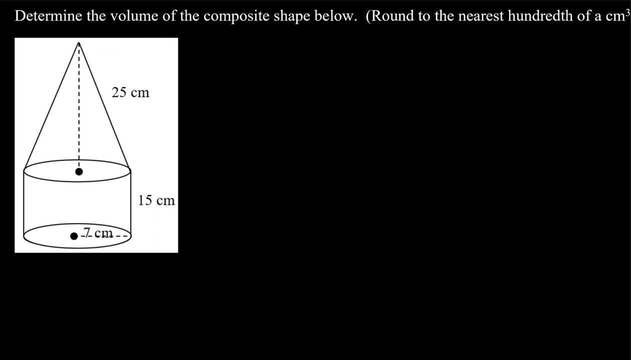 let's try another example: um for volume volume's a little bit easier than surface area. um, i don't really care that this circle on the bottom of the cone and the circle on top of the cylinder are not being presented, so i'm going to try another example: um for volume volume's a little. 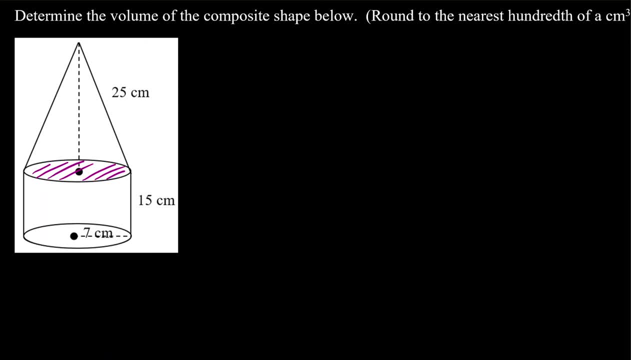 bit easier than surface area. um, for volume, volume's a little bit easier than surface area. the volume- all we have here, the volume of this object, is just the volume of the cylinder plus the volume of the cone. so it's just whatever the cylinder is and the cone together. so the volume. 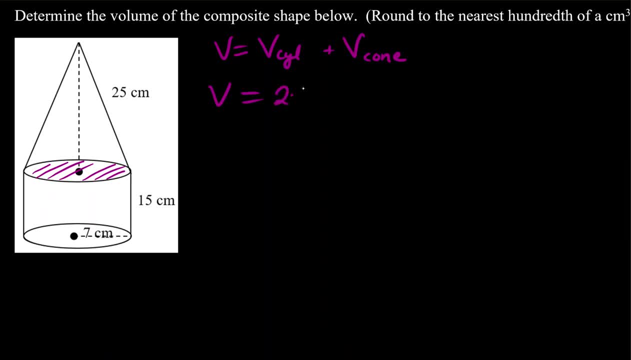 of the cylinder is going to be two- sorry, it's pi? r squared h- and then the volume of the cone is going to be pi r squared squared h divided by three. now we probably should make a little bit of a. we should discriminate between the height of the cylinder and the height of the cone, because 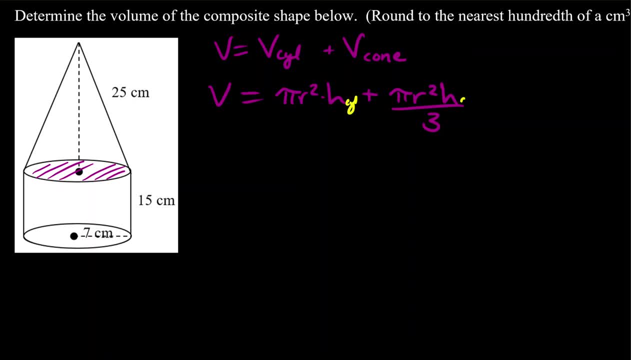 they are two different things. so we'll say height of cylinder and height of cone here, just to be sure. so the volume is pi, the radius is the same either way. it's seven squared and the height of the cylinder is 15 plus pi r. sorry, r is 7 squared and the height of the 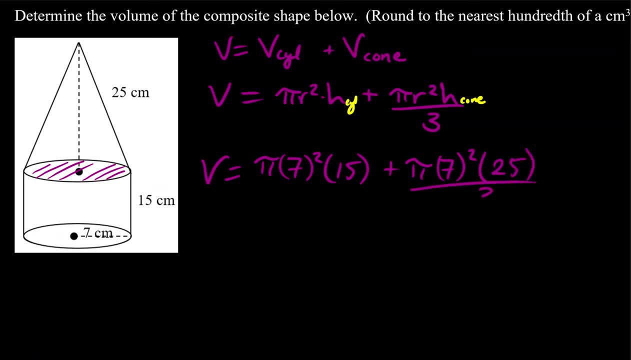 cone is 25 divided by 3. when i calculate this, when i put this into my calculator, i end up getting 3591.88767601. oh, sorry, that's one too many. sevens. 601, blah, blah, blah, blah, blah. and this is centimeters cubed and it says we want to. 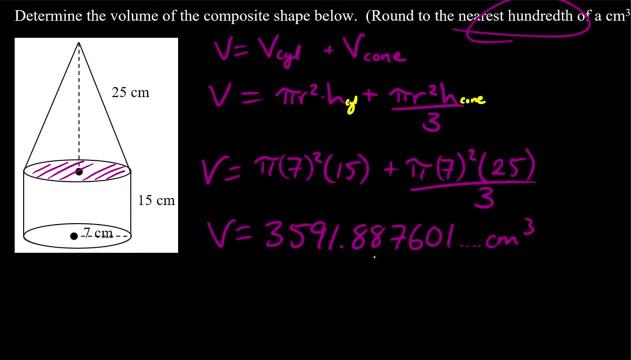 round to the nearest hundredth. okay, we can round to the nearest hundredth. this is our hundredth right here, and since the next digit is a five or higher, we're going to have to round this up to a nine: 3591.89 cubic centimeters. 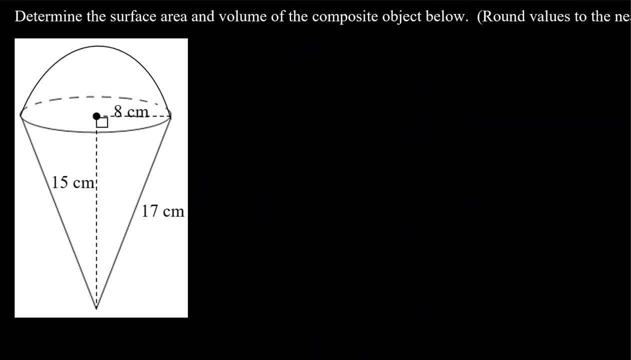 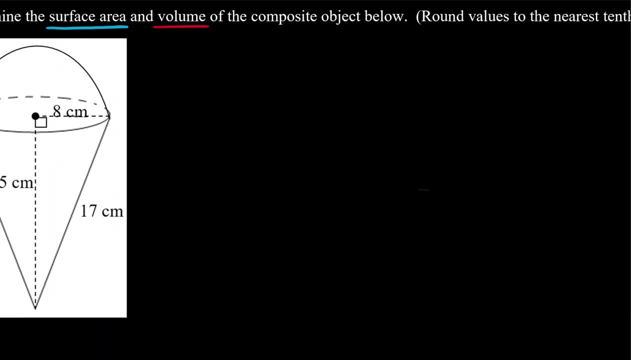 let's try another example. let's determine the surface area and the volume. so we will do the surface area and blue and the volume and red determine the surface area and volume of the composite object below. round the values. you can't see it. it says to the nearest tenth, no problem, so we'll round to. 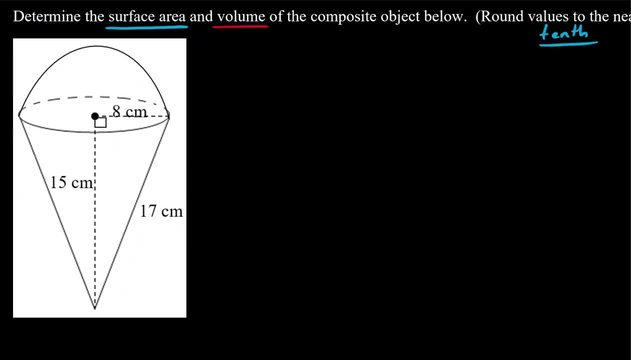 the values to the nearest tenth is what it's saying. so let's try this out. the surface area of this object is going to be the outside, the lateral area of the hemisphere plus the lateral area of the cone. so those are the two sides being presented to me. the surface area is the area of 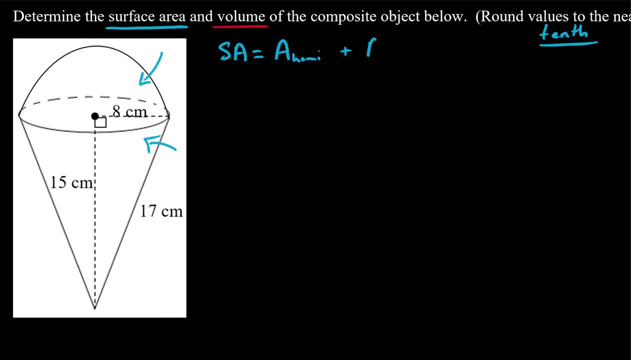 the hemisphere being presented, plus the area of the cone that's being presented. so so, so, so, so so. the hemisphere is just half of a sphere. so instead of 4 pi r squared, it's going to be 2 pi r squared, and then the area of the cone. we're we're wondering: okay, is it the pi r squared or is it the pi r s? 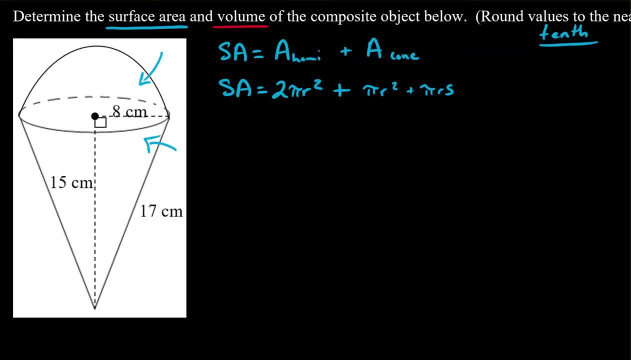 that we're thinking about, and it's. it's definitely not the pi r squared. so that is not the section, because the pi r squared would be the circle on the top of the cone and the circle on the top of the cone would be the circle on the top of the cone. 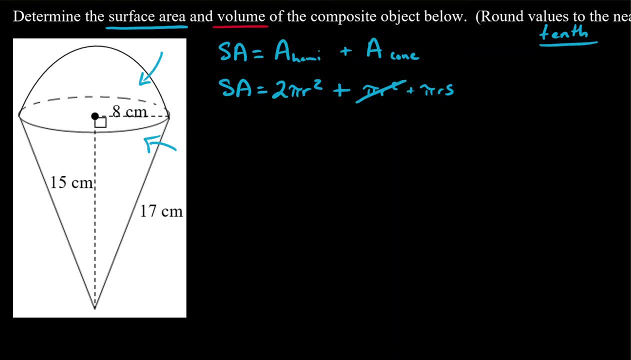 but we don't care about that because it's being hidden by the hemisphere. so the surface area is 2 pi r squared. okay, 2 pi r is 8 squared, and then the lateral area of the, so that's the area all the way around. this cone is high are, which is 8th, and the slant height. the slant height here. 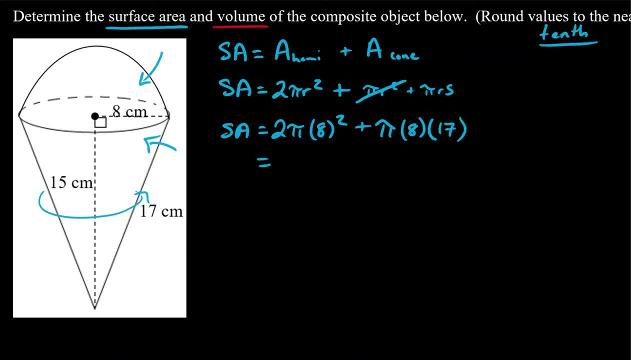 we're telling us 17 centimeters cmr, also called the cone, which is you have an area here and so this plane will be the segment at 8, so it's going to be the CゲP and shit. So when I plug that into my calculator I end up getting 829.3804, blah, blah, blah, blah, blah. centimeters squared. 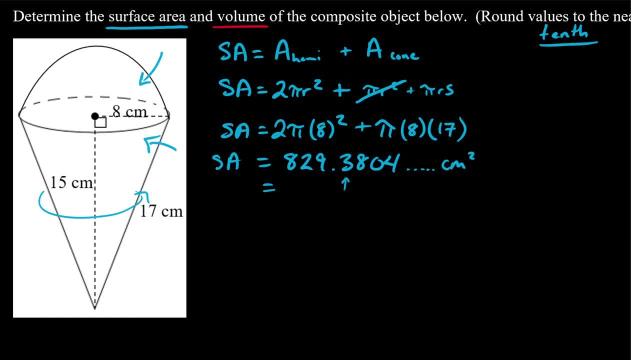 So if I want to round to the nearest tenth, that 3 is going to the 8, sorry is going to make the 3 round up to a 4.. So we end up with 829.4 centimeters squared. 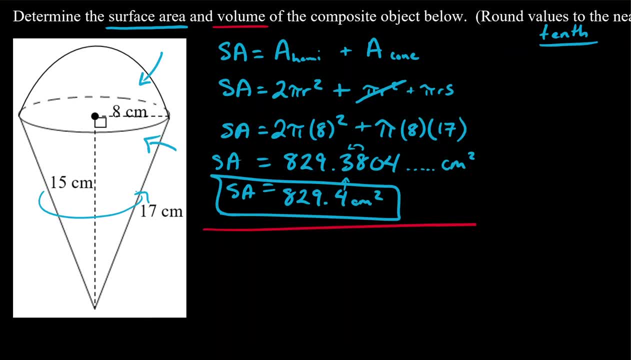 Now let's try for the volume. The volume of our kind of looks like an ice cream cone, I guess- is the volume of the cone plus the volume of a hemisphere. So the volume is going to be the volume of the cone plus the volume of a hemisphere. 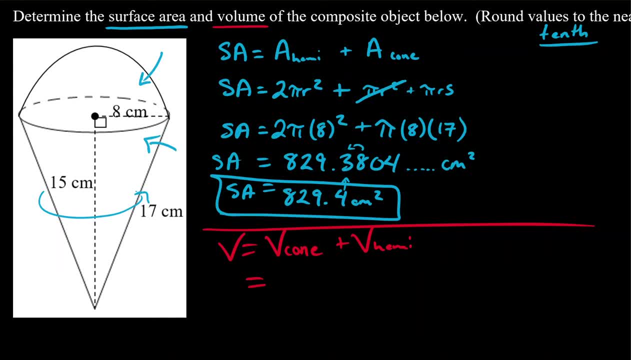 The volume of a cone is, if you recall back to one of our last videos, it's pi r squared h divided by 3.. And then the volume of the hemisphere is half of the regular volume of a sphere. So that's two-thirds pi r cubed, two-thirds pi r cubed. 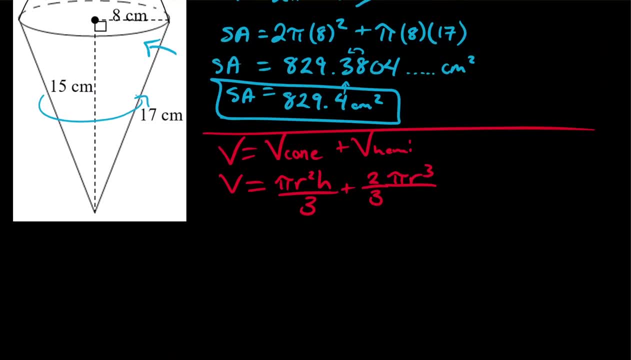 So we can try this out. Hopefully that won't be that big of a deal. Volume pi r is 8, so 8 squared times the height of the cone, that's 15 centimeters divided by 3.. And then two-thirds pi and then the radius cubed. sorry. 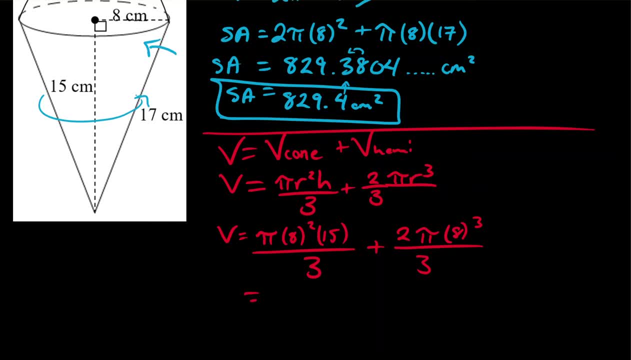 When I punch this into my calculator I end up getting a volume of 1,139.3509, blah, blah, blah, blah centimeters cubed Again. we want to round to the nearest tenth, So the 5 is going to make it round up. 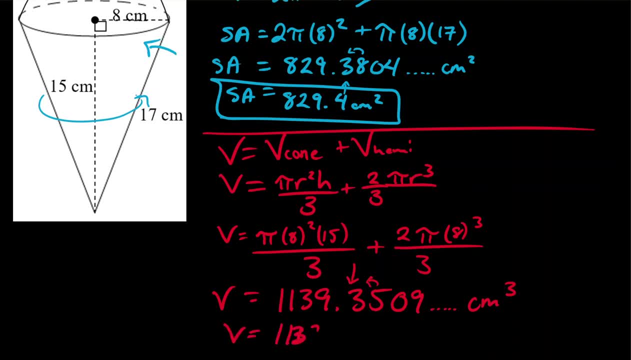 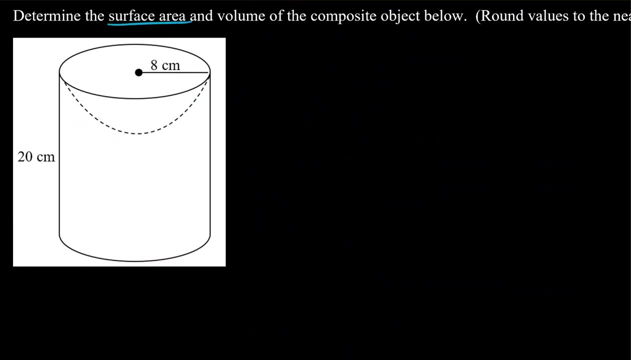 So our volume will be 1,139.4 cubic centimeters. And then our last example. it says: determine the surface area: Okay, we'll do surface area in blue again And the volume: okay, we'll do volume in red. 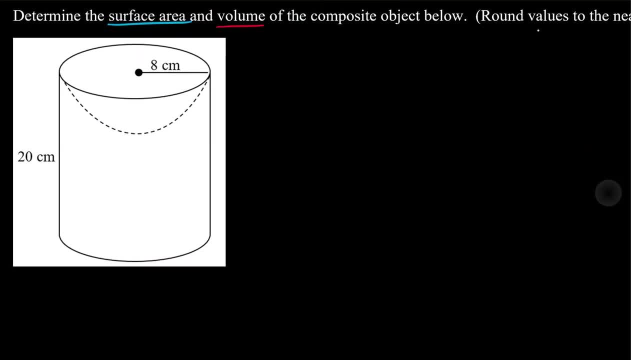 And it says, round our answers to the nearest tenth again: No problem. So the surface area. well, what surfaces do I have being presented? It looks like we have a circle on the bottom That's going to be pi r squared. It looks like we have the lateral area of the of a cylinder- no problem. 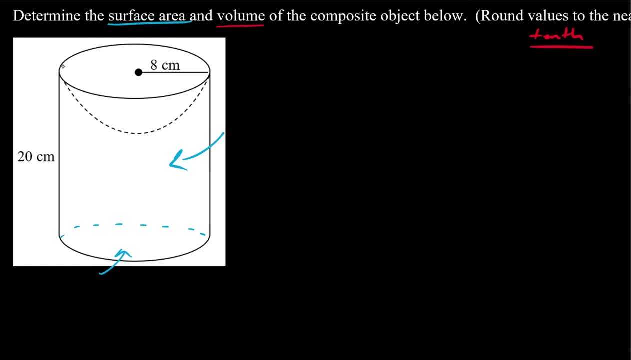 And then we've. it's almost like we have a scoop cut out in the shape of a hemisphere, And it doesn't matter if it's cut out, because that surface of the hemisphere is still being presented to us. So the surface area of this object is going to be the hemisphere. 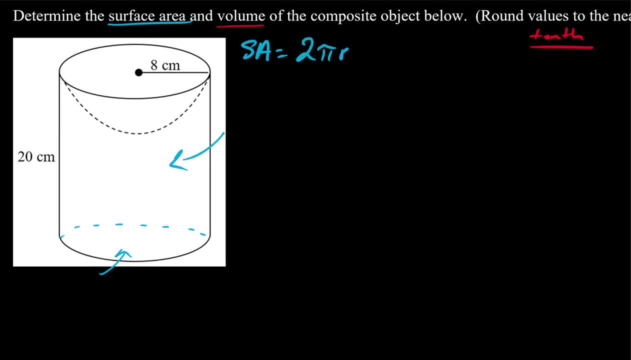 Well, that's half of a sphere, So that's 2. Pi r squared plus we have the sphere, the circle on the bottom, So that's pi r squared plus we have the lateral surface area of a cylinder. So that's that all the way around bit. 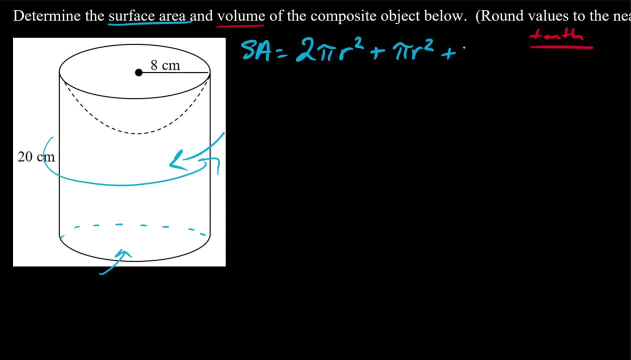 And that is, that is 2 pi r h. Okay Well, 2 pi r squared plus pi r squared is really just 3 pi r squared, pi R squared. so that'll give us a little bit of reprieve from our calculation 2. 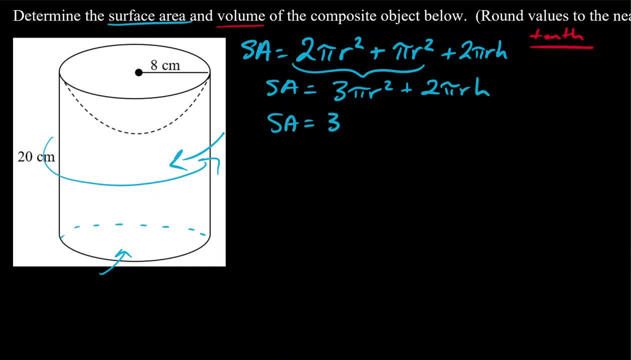 pi Rh. so the surface area, 3 pi- we know R is 8 squared. and then 2 pi R is 8. again, the height is 20. so when I put this into my calculator, the surface area, I end up getting, and we want to round it to the nearest tenth. so one, six, zero, eight point four, nine five. 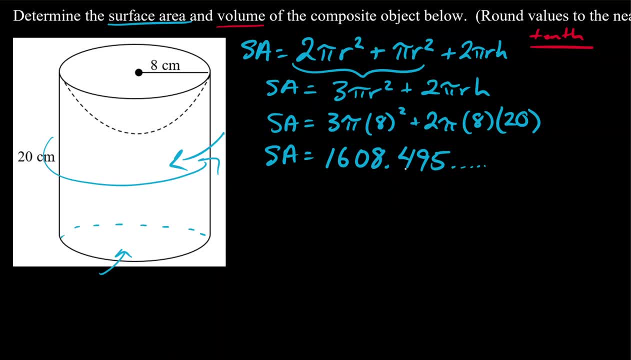 blah, blah, blah, blah blah. the tenth is our four, so our four is gonna round up to a five, so we'll just change that to a five. and this is centimeters squared. perfect, let's try our volume. now. our volume is is the volume of the whole square. 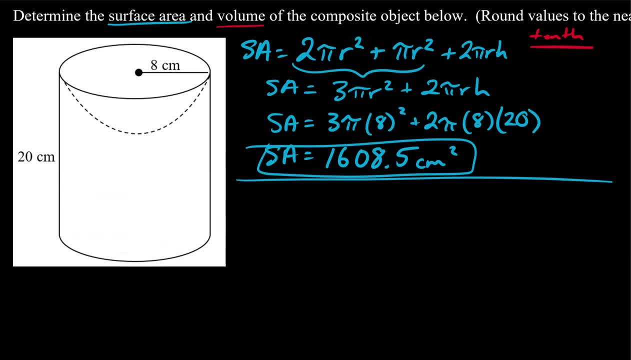 cylinder, but it looks like we've scooped out this hemisphere here, so it's like we're gonna take the volume of the cylinder. the volume total is the volume of the cylinder, and then we've scooped out the volume of the hemisphere, so the volume of a cylinder is 2, sorry,